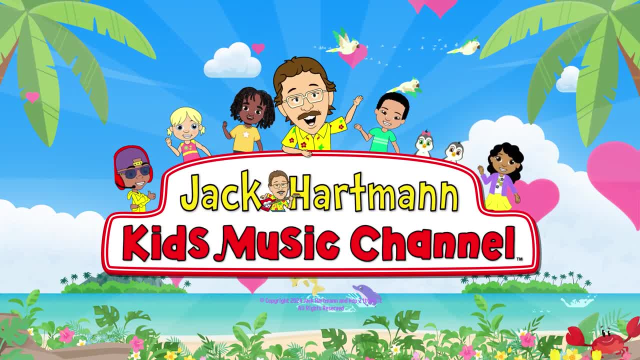 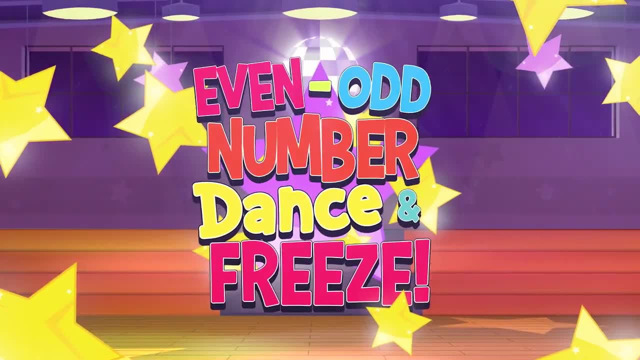 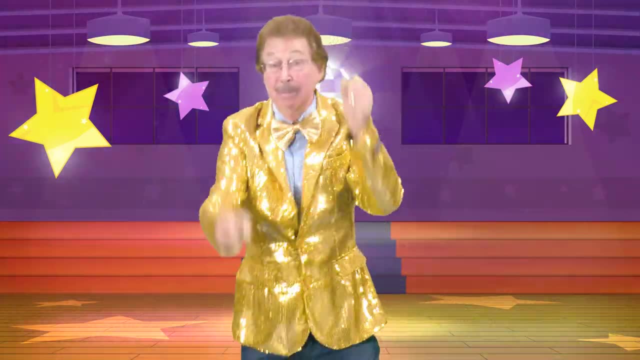 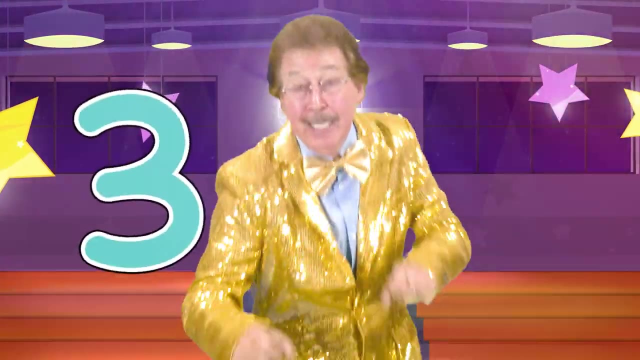 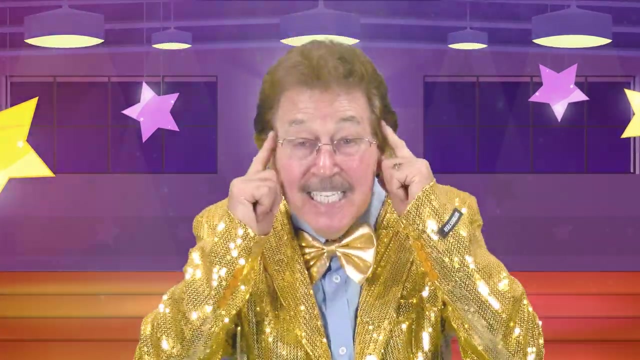 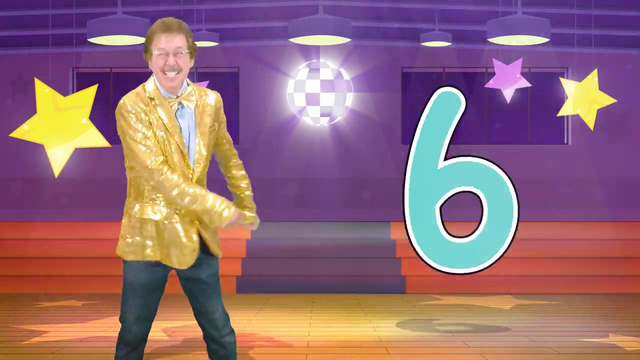 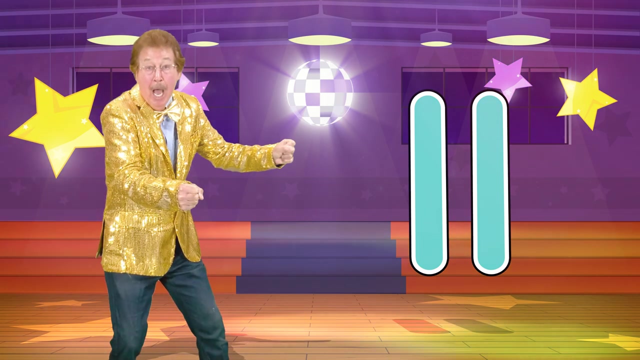 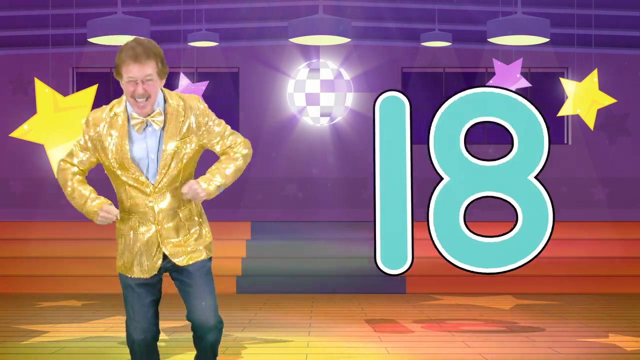 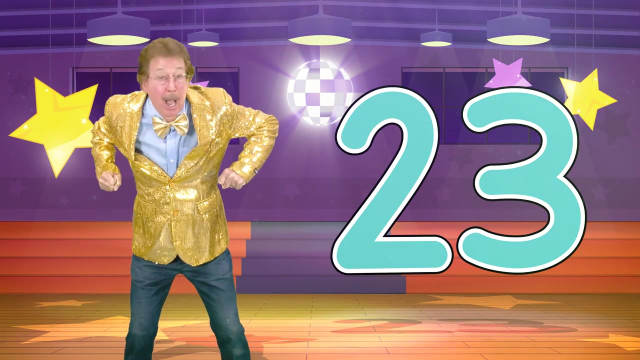 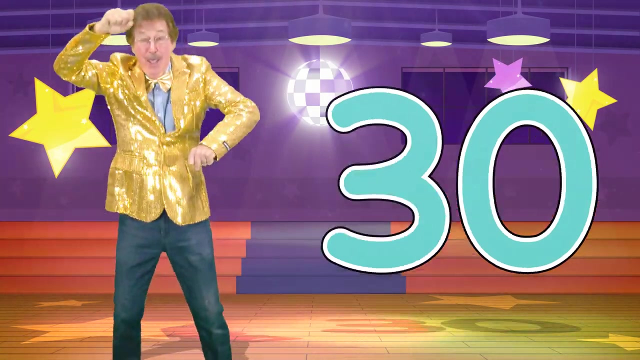 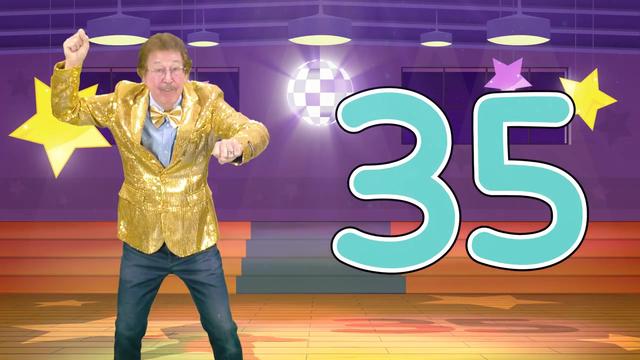 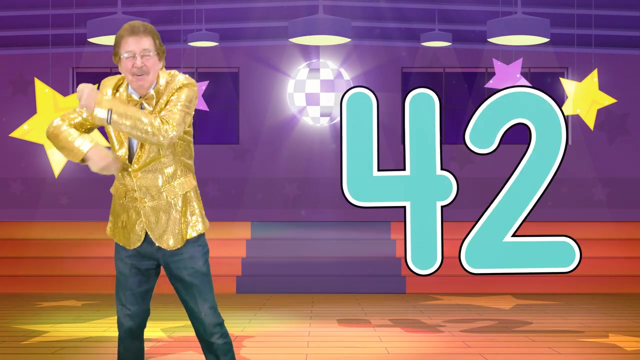 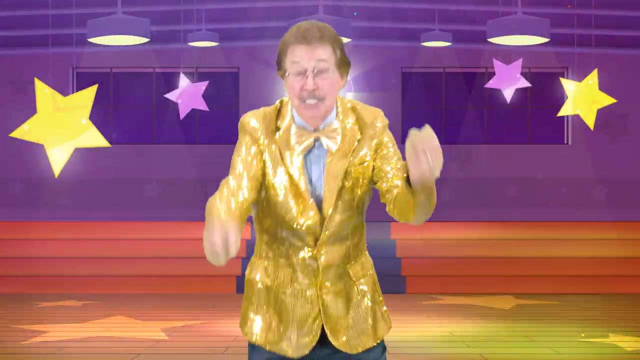 Jack Cartman Kids in the Channel. Please listen and dance. two, four, six, eight, ten, eleven, thirteen, fifteen, sixteen, eighteen, twenty, twenty-one, twenty-three, twenty-five, twenty-six, twenty-eight, thirty, thirty-two, thirty-three, thirty-five, thirty-seven, thirty-eight, forty, forty-two, forty-three, forty-five. Come on dance. 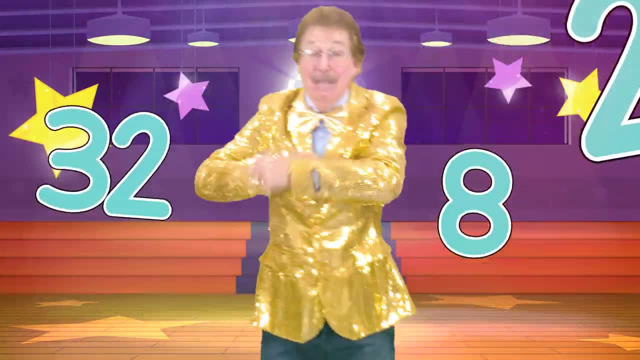 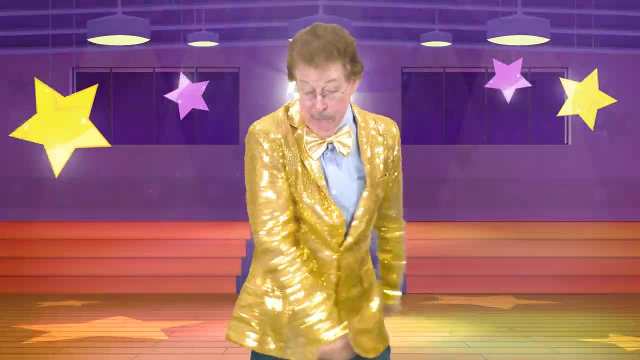 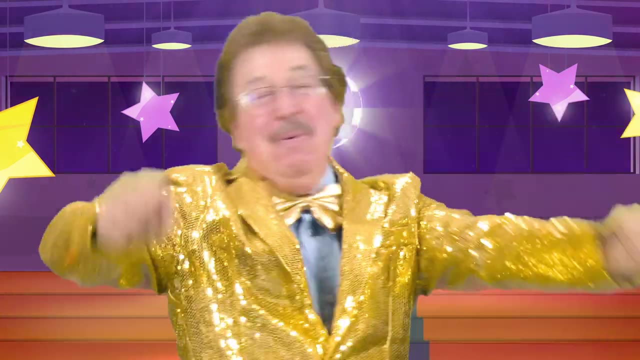 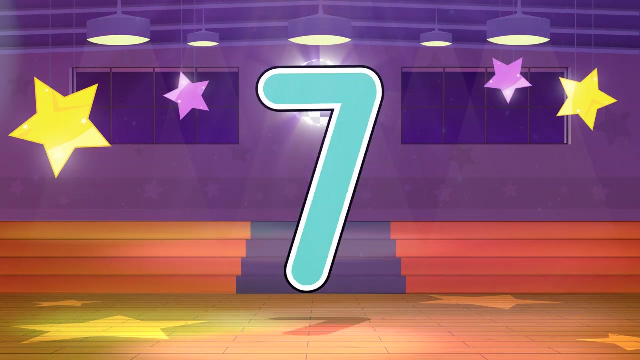 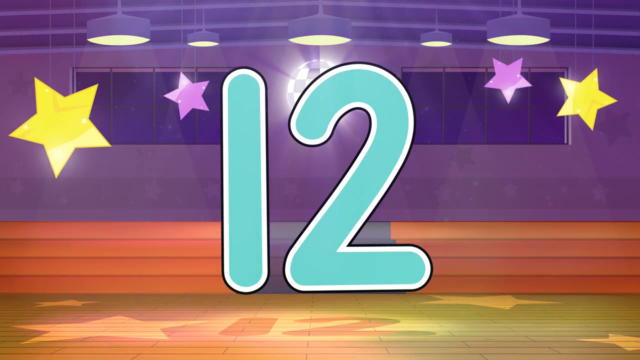 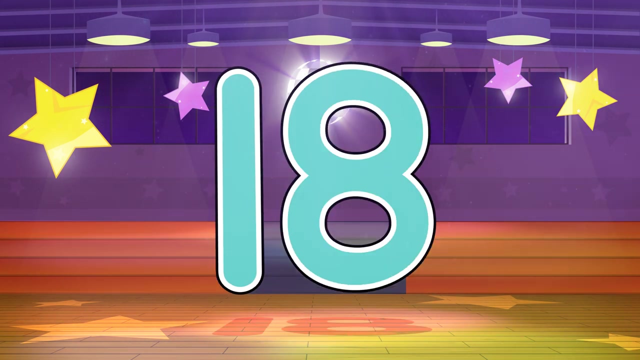 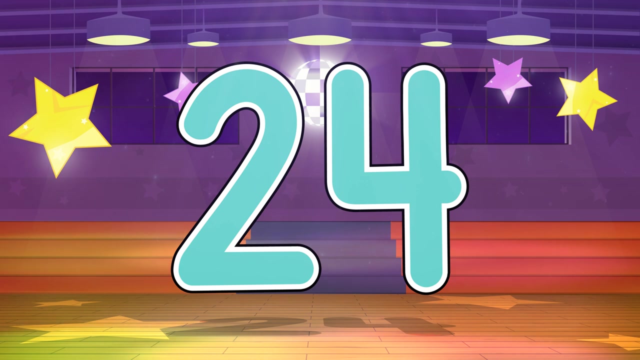 and count with me. Dance on even numbers. Listen carefully. If I say an odd number like three or thirteen, You stop dancing and freeze. Listen and look. Dance on your own. two, four, six, seven, nine, ten, twelve, thirteen, fifteen, seventeen, eighteen, twenty, twenty-two, twenty-four, twenty-six, twenty-seven. 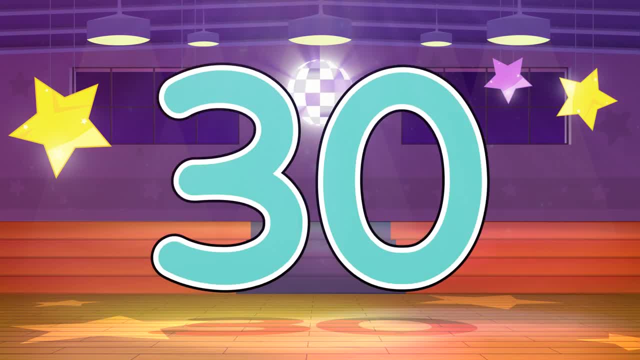 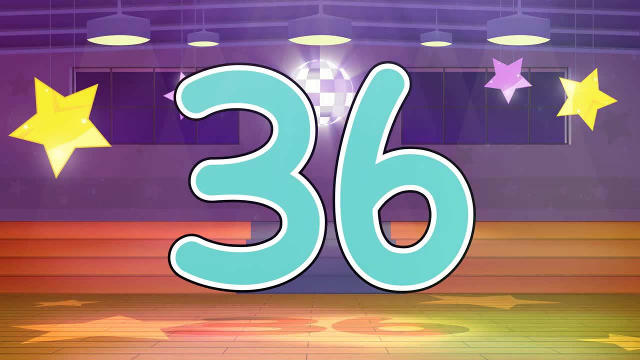 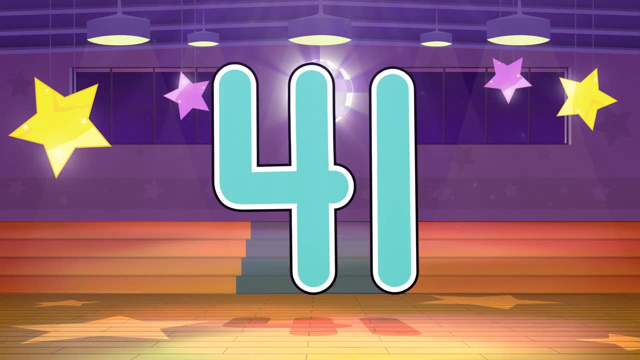 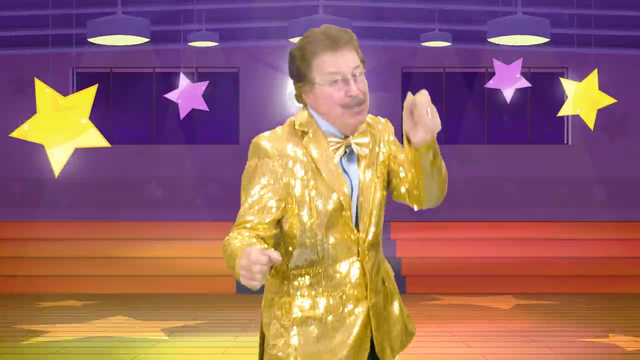 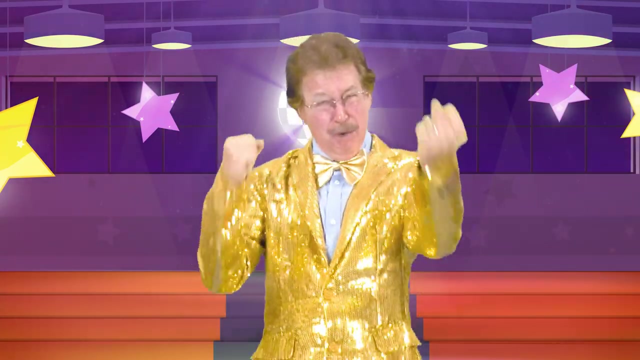 twenty-nine, thirty, thirty-two, thirty-three, thirty-five, thirty-six, thirty-eight, forty, forty-one, forty-three. Wow, math is fun. Math is cool. You danced and did the best that you can do. Your brain and body is getting smart and strong. Keep learning math and keep singing along.